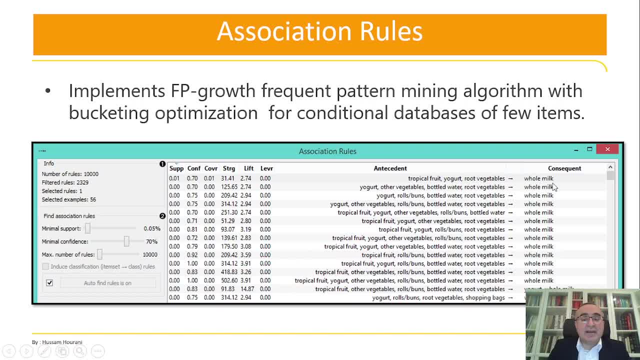 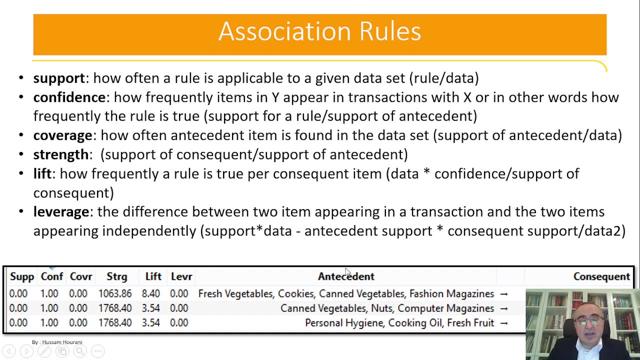 here, most of the people will buy whole milk, So this is a rule. So can you identify all these rules From your data set that you have based on these measurements? the answer is absolutely yes. So to do this, you need to understand these few measures for the rules to happen. 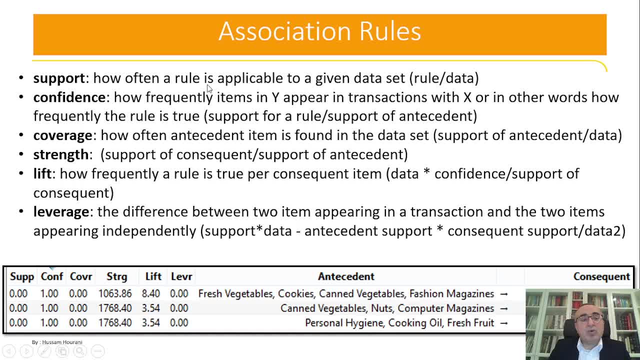 The first one is support. Support is how often a rule is applicable to a given data set. Confidence: how frequent item in Y appears in a transaction with X, or in other words, how frequent the rule is. Coverage is how often antecedent item is found in the data set. 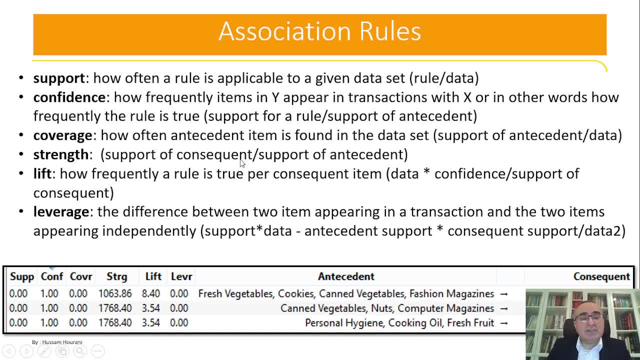 Strength is support of consequent over support of antecedent. Lift is how frequent a rule is true per consequent item. And the last one is leverage, which is the difference between the two items appearing in a transaction and the two items appearing independently. 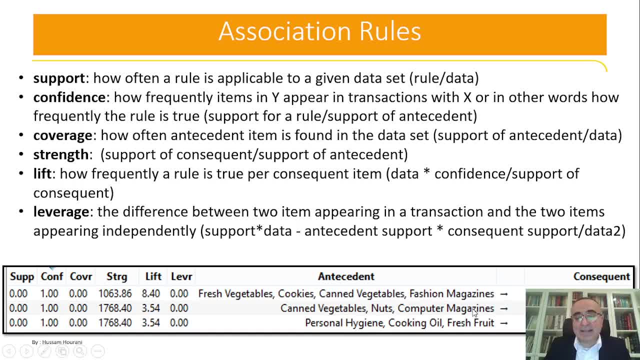 So this is, for example, a simple, simple data set. This is the antecedent and this is the consequent and this is the consequent. So, for example, if we take the second item, if you it identified from your, 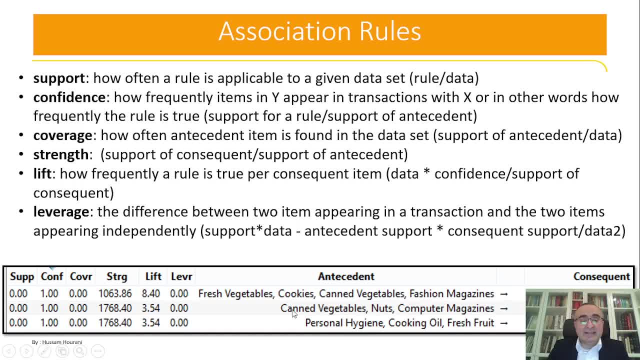 data set that if you buy canned vegetables, nuts and computer magazines, you will buy definitely fresh vegetables, because most of the customers have this habit or have this. you know rule, So we call it association rule. We have antecedent and we have the consequent. 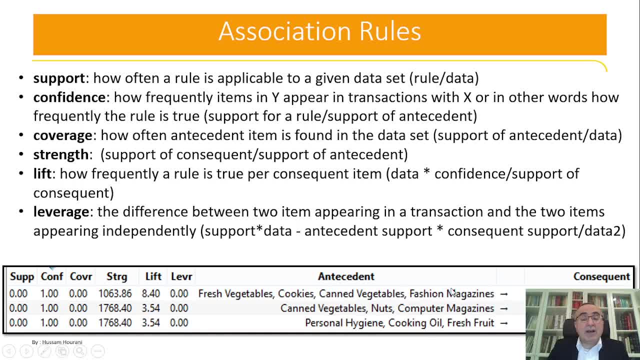 So if you buy something, you will buy something else, And if you identify all these rules, you as owner for a huge supermarket, you will understand that, for example, the there are some association rules between the items that you have in your 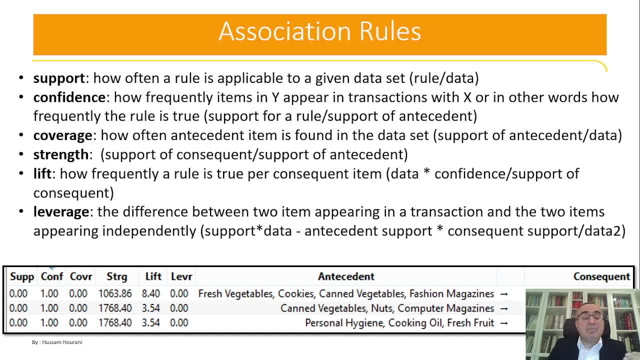 supermarket, So you can always get prepared with the proper numbers of items in your shelves. So this is, for example, the support: zero, the confidence is one, the coverage is zero, the strength is 1768, and the lift is 3.5, and the leverage is zero. 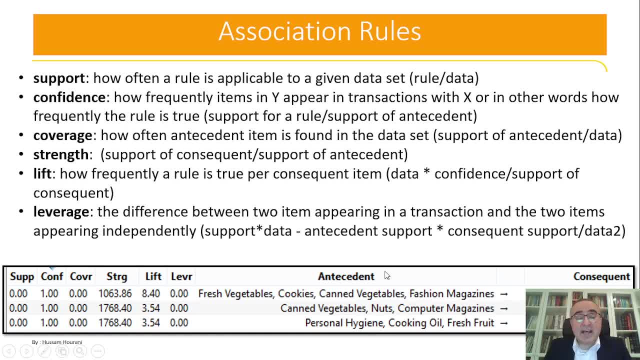 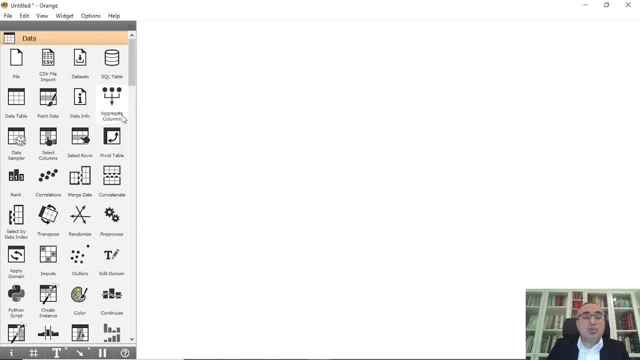 So how to do this in orange data mining. It's actually a straightforward implementation. Let's go into orange and try to do this. So I will use a data set. Okay, I will bring the data set and from data set I will use. 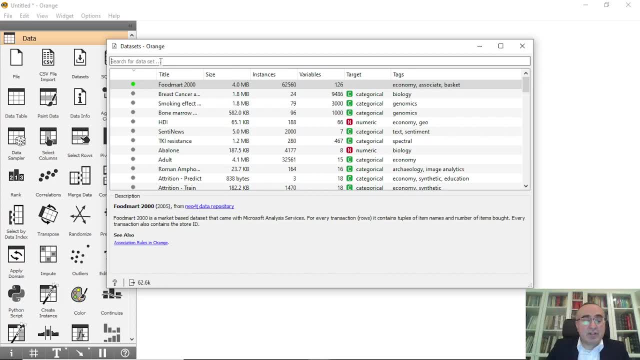 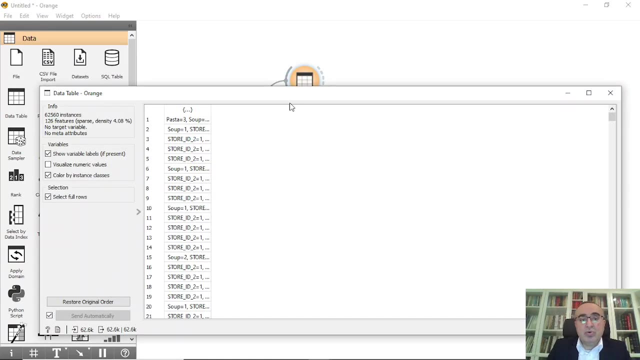 food mart 2000.. You can search for it from here. You can click food, for example, and this is the food mart 2000.. Okay, so if you open this one as a data table, it will bring you this data set. 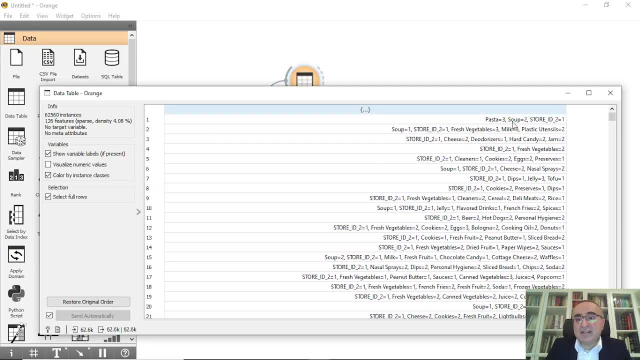 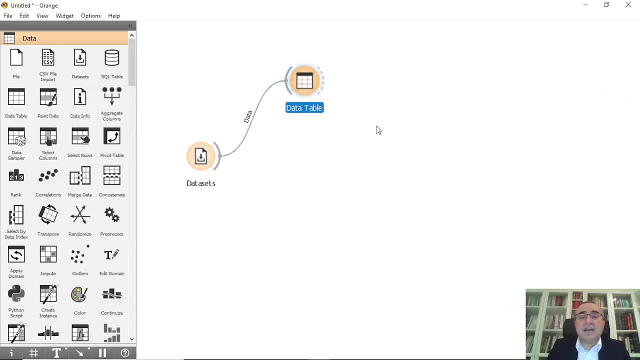 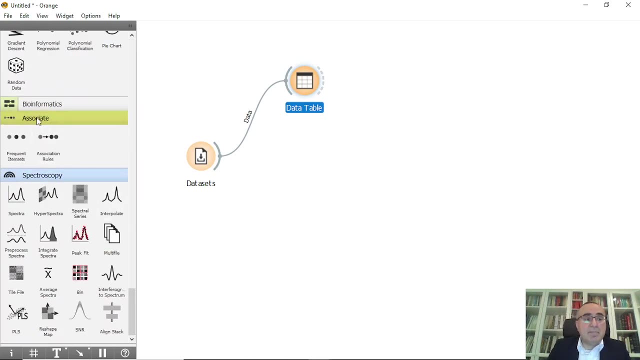 Okay, so these are the items and number of times you purchase these items. So, from all these items, can you identify them? Can you find the association rule? The answer is absolutely yes, What we will do. we will use the associate panel. 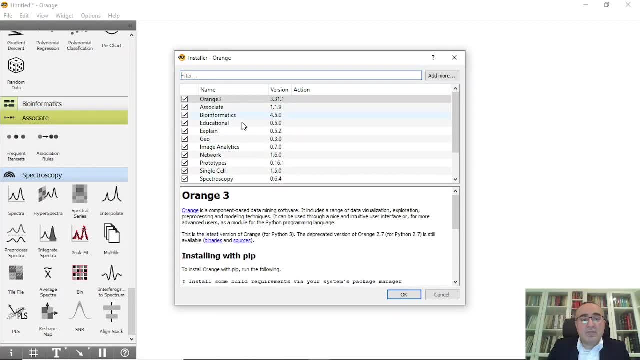 This is the associate panel. You can download it from here, from ads on, and you can go into associate. This is the associate. You can click on it and you can click OK till you install it and then you reset your application and it will appear here. 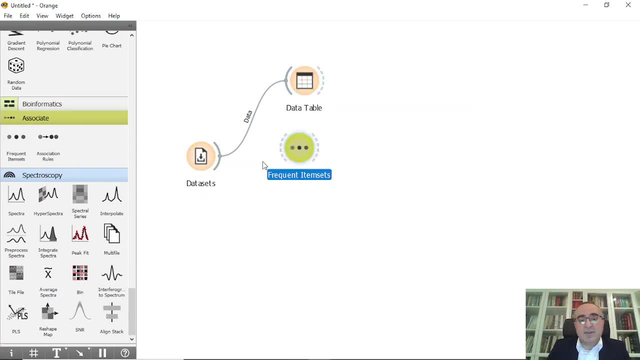 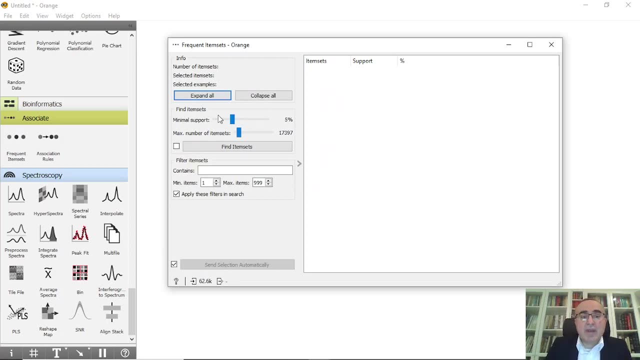 So the first one I will use is the frequent item- frequent item, So I will connect this data set To this frequent item and from the frequent item, if you double click, you can identify items based on the minimum support and maximum number of items. 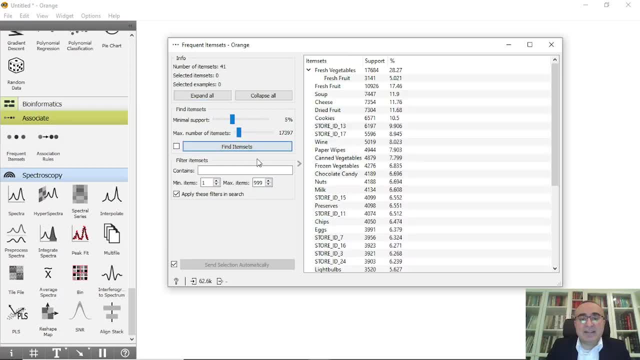 You can identify this, So you click, then find items. You will identify all these items based on your criteria. So this is, for example, the fresh vegetables, and your data set is 17,684.. And, for example, the fresh vegetables. 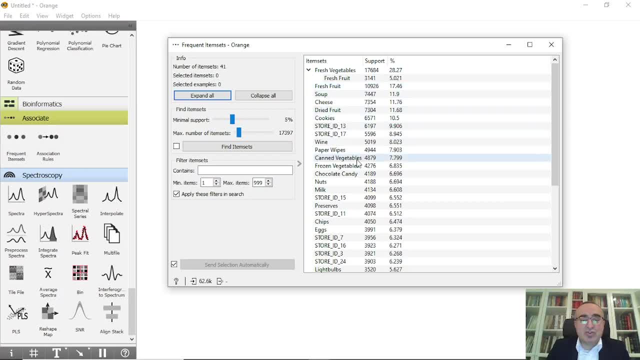 Okay, Uh, fruit is 10,926, and so on and so forth. So this is the first one. You can identify how many items appears in your data set based on the rules you associated or based on the criteria you set here. This is the first one. 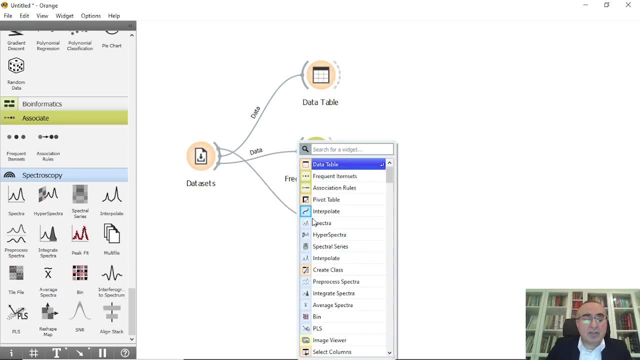 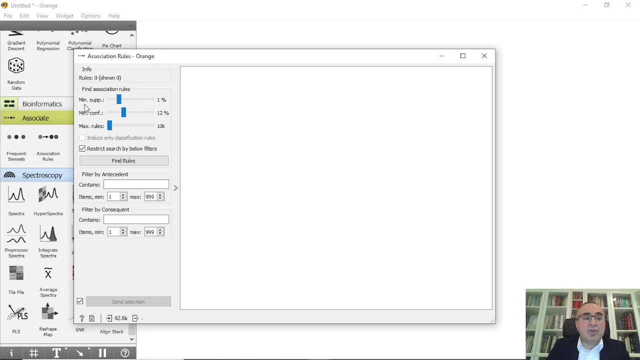 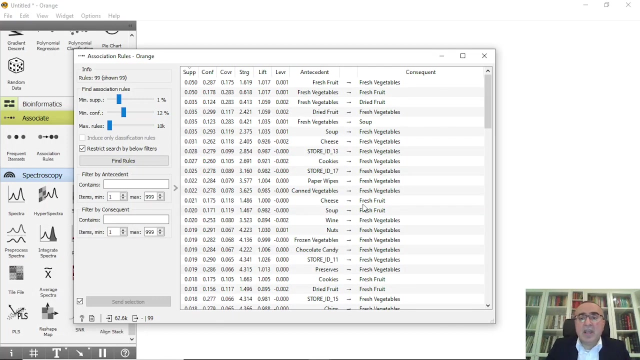 The second one is you connect this to associate rules. which is this one here? associate rules, Okay, And from associate rules, you double click And You first identify your criteria, uh, your association criteria, for example, the minimum support, minimum confidence, maximum rules, whatever you can put, uh, you can increase, decrease, whatever you want. and then you click find rules and, based on five rules, it identify all the rules in your data set. 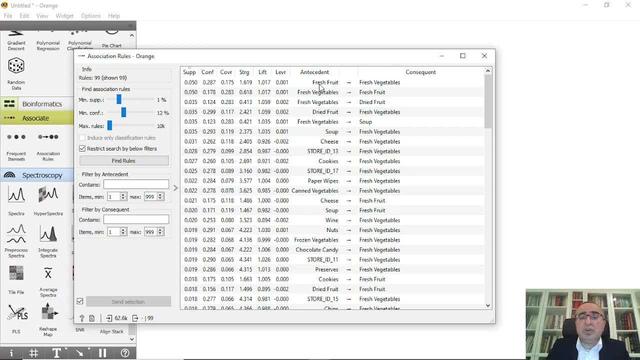 For example- let's take the first one- fresh food. If you buy fresh, fresh food as antecedent, you will definitely, uh, uh, not maybe definitely as definitely, but uh, you will most likely buy fresh vegetables. based on this confidence, based on the support and coverage and sync and lift and leverage, 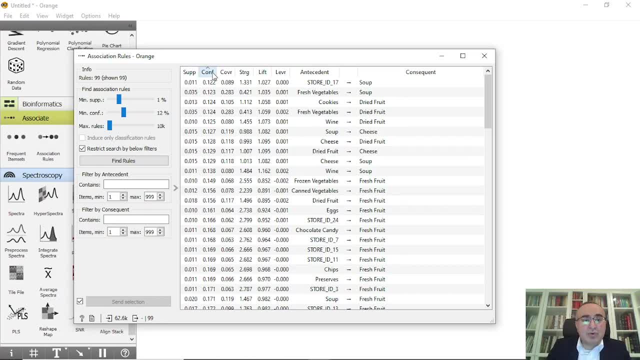 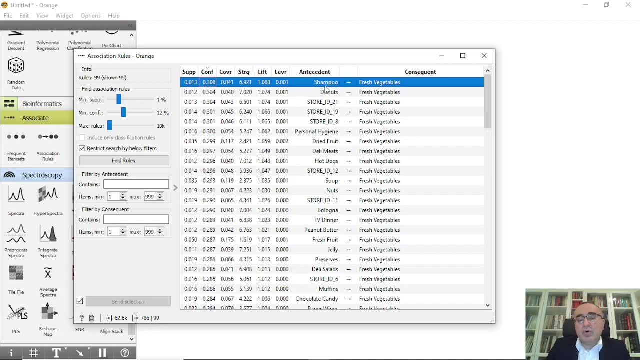 These are the numbers. For example, if you click here the most you know the. this is the most uh frequent maybe item. The first one is: uh, if you always buy shampoo, then you will uh buy fresh vegetables. 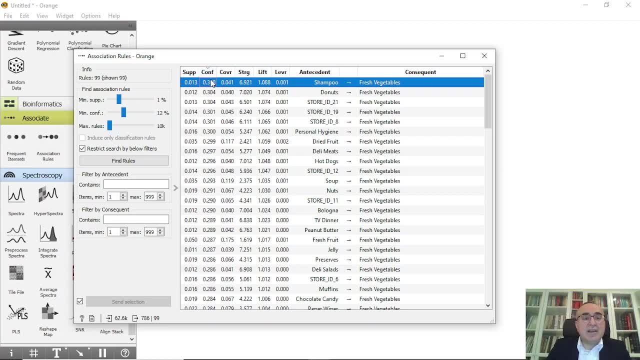 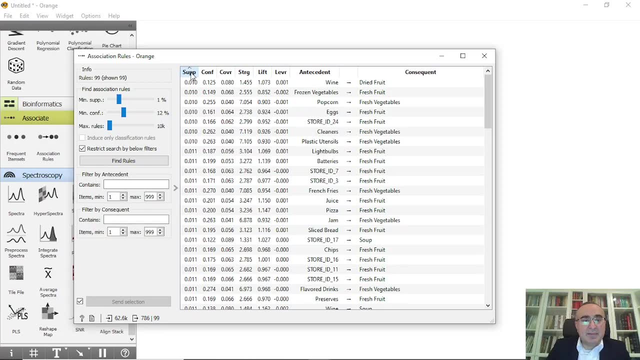 For example, it has uh 0.3. Confidence and the support is 0.013.. If you click in the support to get the most uh items, maybe this is the item If you buy from support perspective. if you buy fresh fruit, you will buy fresh vegetables, and so on and so forth. 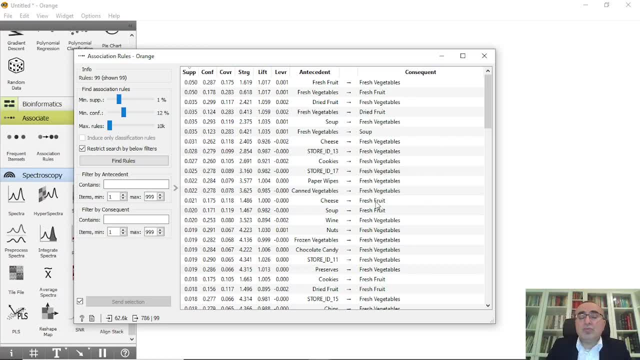 This is actually very important for the people: to find some rules in the data. Remember, we're not talking about features, We're talking about the data itself. We need to identify The rules from the data that you have. this is exactly what's happening. 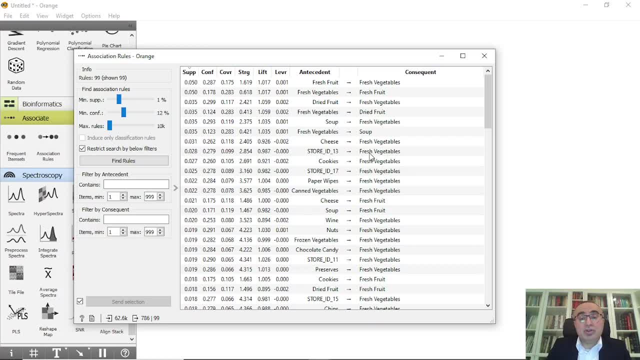 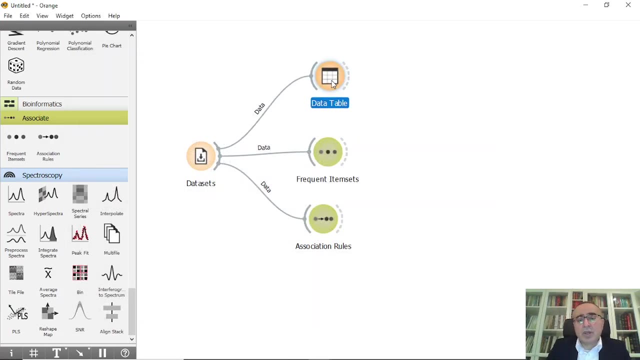 And, um, the people who are looking for a solution for their problems will definitely go into this because they wanted to see all the association rules between their items, as you can see from here. So this is a very important subject. I wanted really to show it to you and show how you do this. 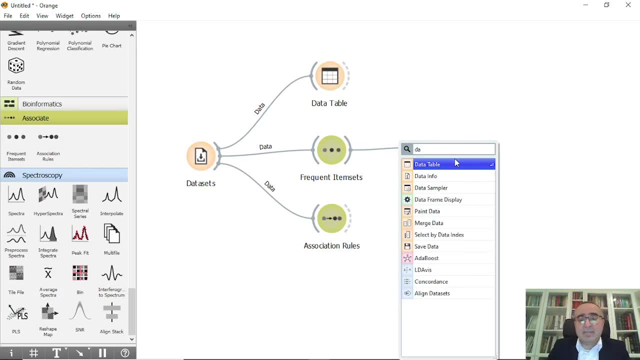 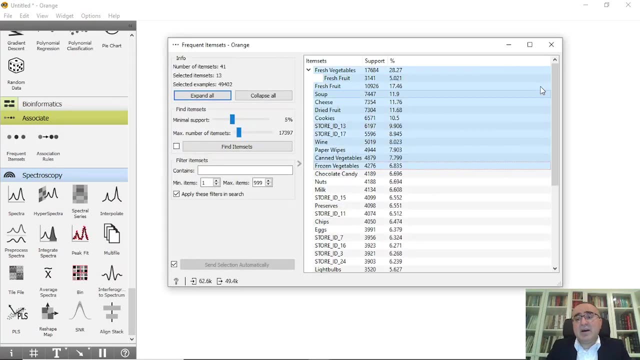 It's as simple as this and also you can connect this to data table, Okay, And you can Extract, for example, the uh match items. So you can select, for example, these items and you can then uh print them here.